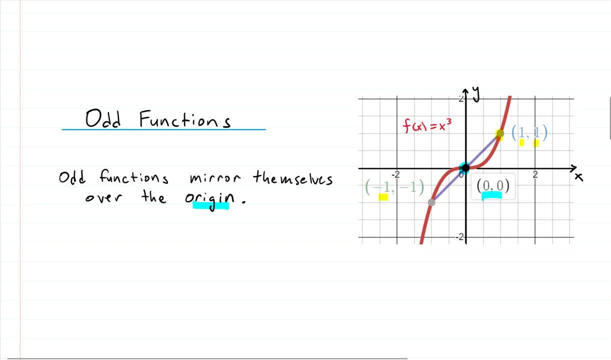 take the opposite of the sign, which would give you a negative 1. negative 1, that point will also be on the curve and you can join those two curves- or, sorry, excuse me, those two points, with a line that will pass through the origin. so this is a characteristic, it doesn't matter which. 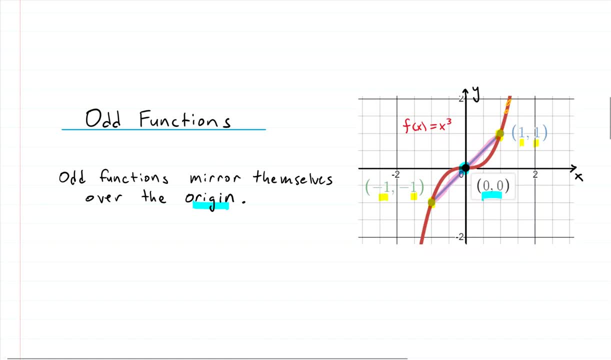 point you pick. you could pick any point up here in quadrant 1 and you would be able to find the corresponding point in quadrant 3. this is quadrant 1 and this is quadrant 3. in case you're wondering, you'll be able to find the. 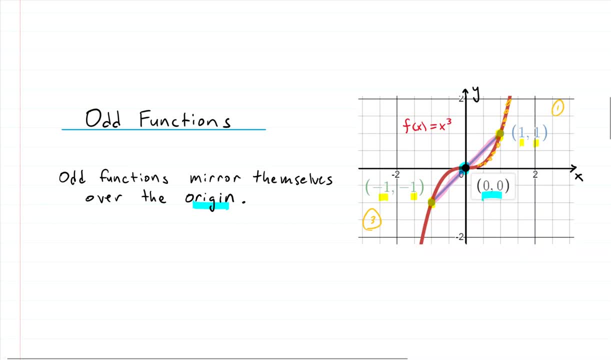 corresponding point in quadrant 3. that is the opposite sign, and you can join those two points with a line that passes through the origin. so the this type of really cool symmetry through the origin defines an odd function. if your function has this type of symmetry, then your function is an odd. 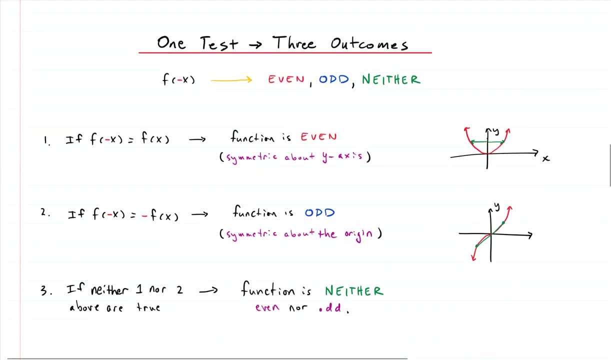 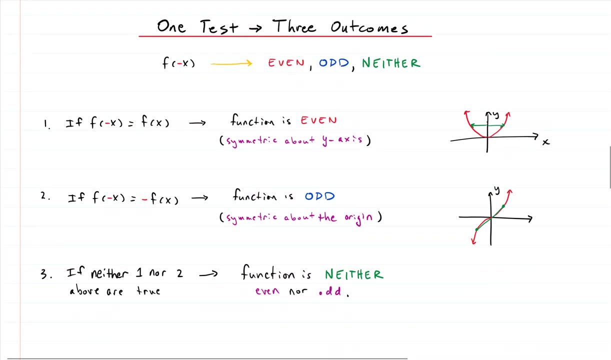 function. let's talk about the one test to rule them all. sorry, I couldn't resist that. one test, three outcomes, so the test is actually pretty simple. all you do is you plug in a negative x instead of an x into your function. you simplify and you see what you get. 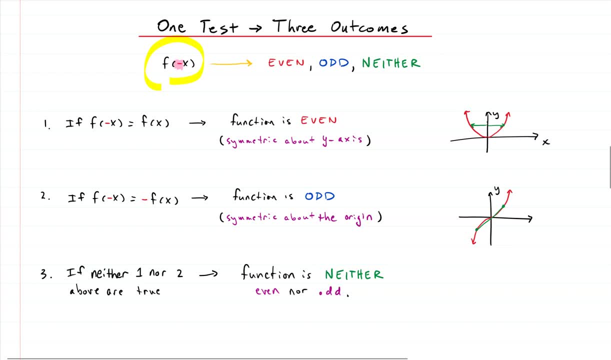 out and what you get out will tell you whether or not you have an even odd or neither of those two. so pretty cool, huh. if you take a negative, look at the test for even functions. if you take a negative x and plug into the function that you're given and you get out exactly the same function as you had to. 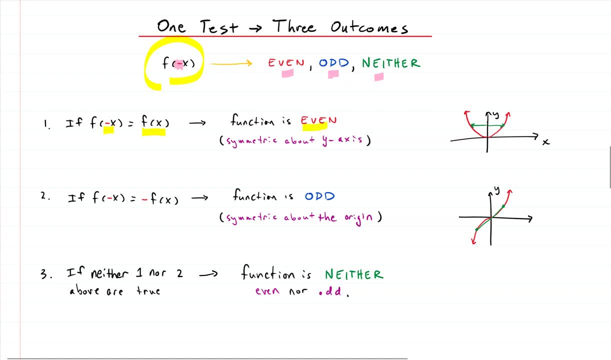 begin with, before you put the negative in. then you have an even function, which means you have symmetry about the y-axis, which can be seen here in the beautiful graph. If you put the negative in to the function and you get back the original function, 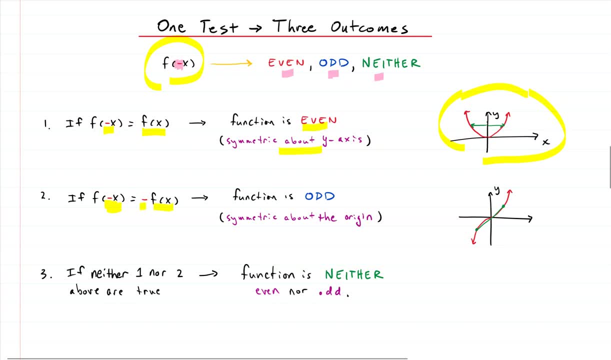 but multiplied by a negative, so the negative of the original, then you have an odd function. If you don't get back either the function itself, which is in case one, or the negative of the original function, which is case two, then you know that you are in the neither category. 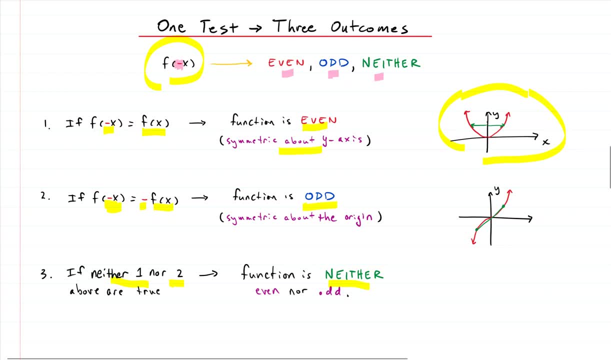 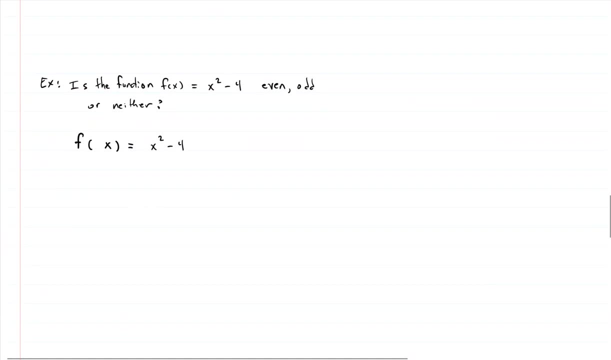 and the thing that you have is neither an even nor odd function. Let's try these out. We have an example for each of these, so let's see how this works. So the question is: is the function x squared minus four even, odd or neither? 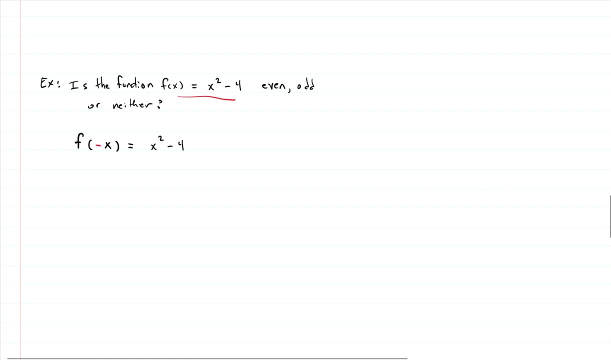 So we have our function down here. If I put in a negative instead of the x and then we simplify, we can see what happens And what does happen. Negative x, quantity squared just gives us x squared and the negative four stays the same. 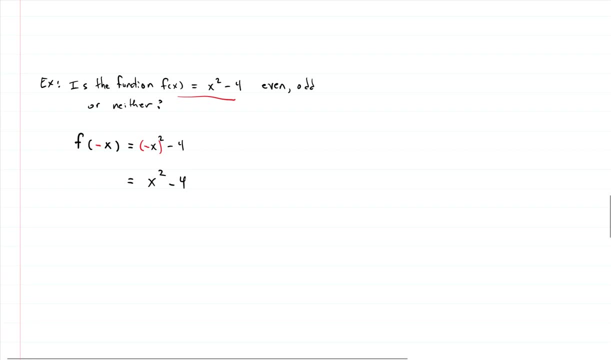 So what is that? Is that the exact same thing that we got back? It is actually That's the original function, right? Because the original function was x squared minus four. That's exactly what we have: x squared minus four. 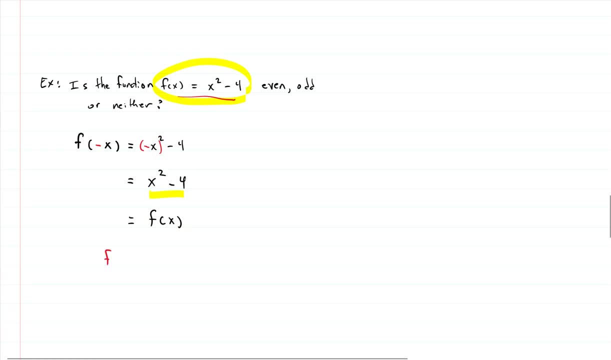 So we plugged in. we plugged in negative x and we got back the original function. So this function we're dealing with, x squared minus four, is an even function. Let's try another one. So our original function then now is x cubed minus x. 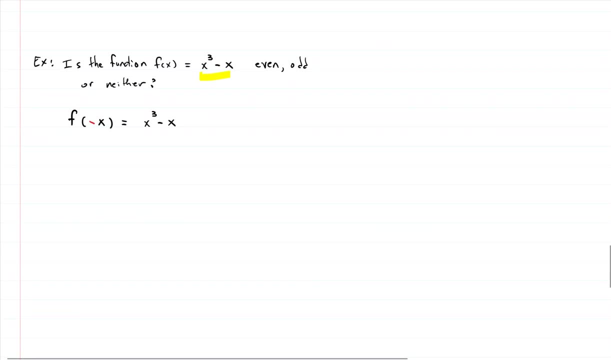 So instead of having an input as an x, we're going to input a negative x. So that means we have a negative x here and we have a negative x there. Now we just do some algebra. We simplify Negative x, cubed negative times. negative gives us a positive. 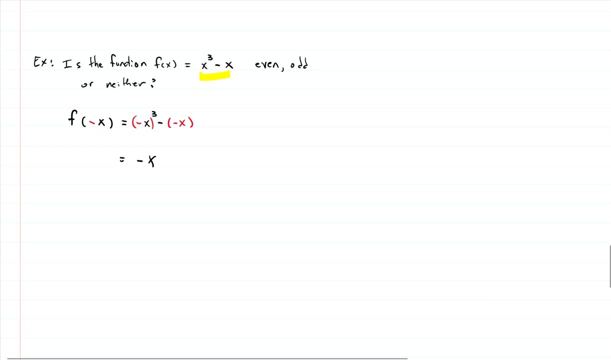 and then times a negative again gives us a negative. So we have negative quantity x cubed and a negative and a negative. this negative distributed gives us a positive x squared, And we look at that and we're like, hmm, is that the same? 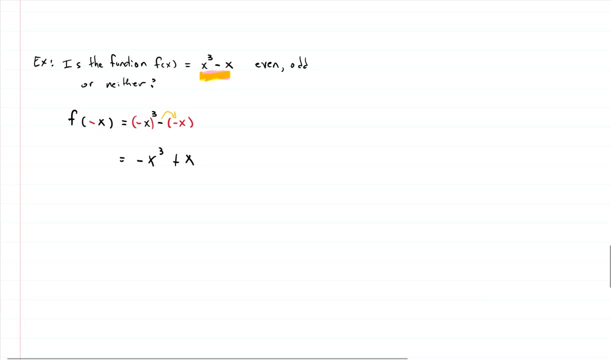 as the original. The original again was x cubed minus x and the signs don't match up. but let's factor out a negative and see what we get. So if we factor out a negative, what do we have left? We have x cubed and then we have a negative x there. 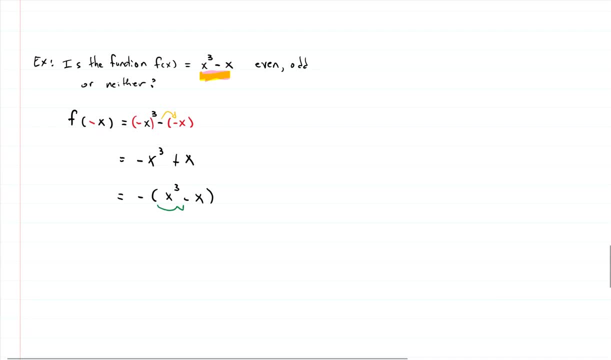 And we look at that and we're like, hey, check that out. What is this right here? Well, that's the function itself, right? So we got back the negative of the function. So we plugged in the original equation: negative x. 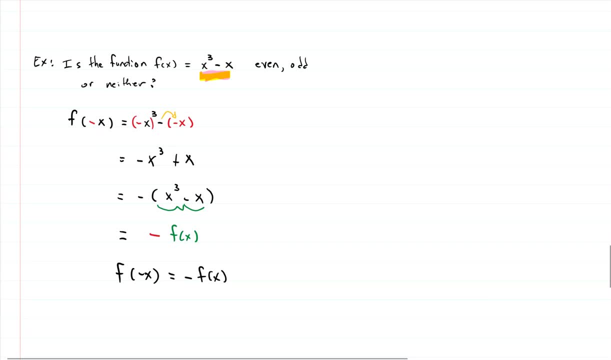 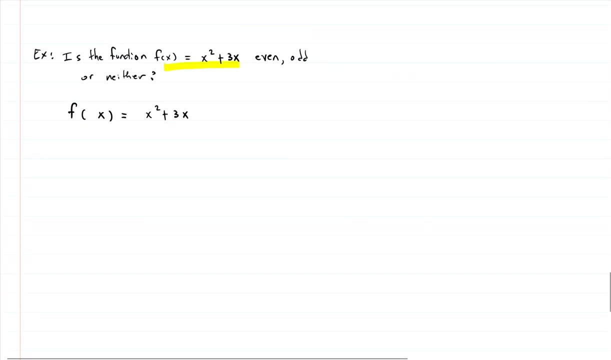 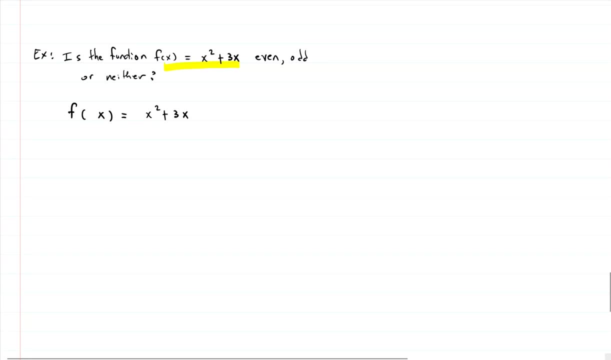 Or neither of those two. So again, the first thing we do is we take the function and we, instead of plugging in x, we plug in a negative x. So we have a negative here and let's put in a negative here for this x. 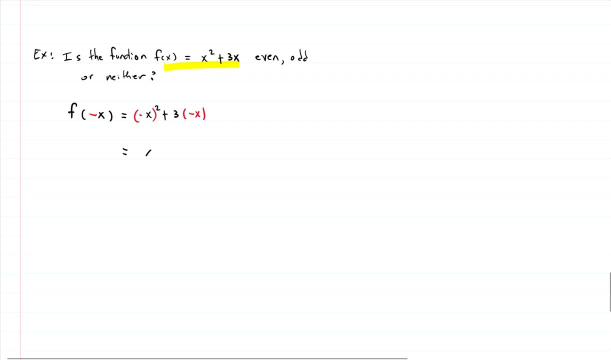 And now we just do some simplification. So negative x squared gives us x squared And the negative in the 3, give us negative 3x. So we're done simplifying and we look at it and we say: is this the same as the original? 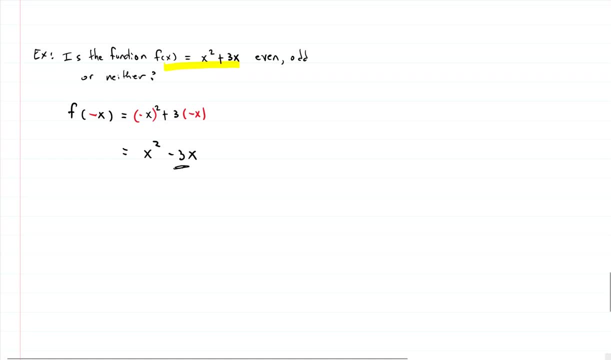 The x squared's the same. but then we have a negative down here but we have a positive up here in the original. So it's not the same. So let's see, if we factor out an x, if that changes anything. If we factor out an x, we get a negative x squared. 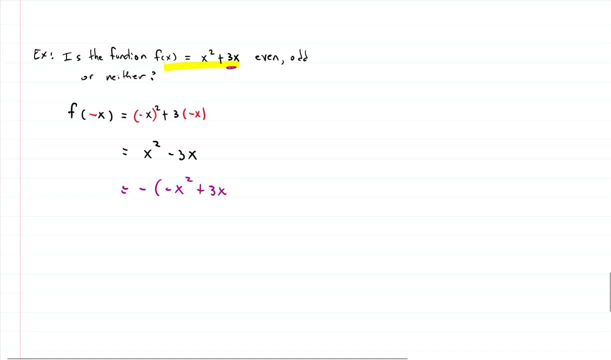 and a positive- whoops, a positive three x. Is it the same now? Well, the three x is now the same as the three x, but now we have a negative x squared in our simplified one. but we don't have that in the original. 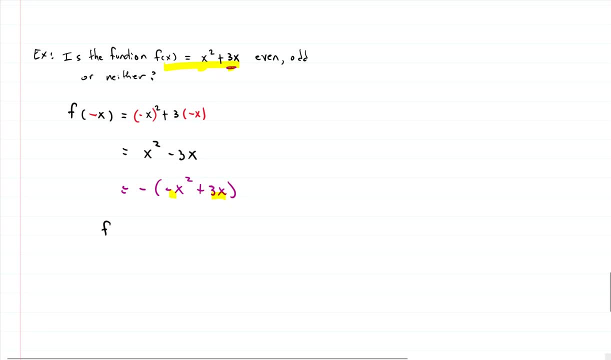 So it's not. once we plugged in the negative x into the function, it was not the original and it was not the negative of the original, So our function is neither even nor is it odd. Hopefully this video was helpful and gave you some background.